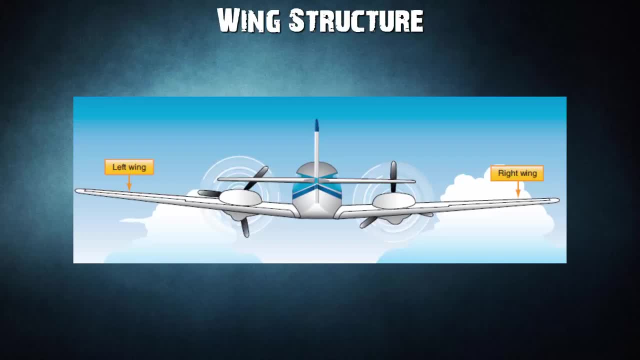 The wings of aircraft are designated left and right, corresponding to the left and right sides of the operator when seated in the cockpit. Often wings are of full cantilever design. This means they are built so that no external bracing is needed. They are supported internally by structural members assisted by the skin of the aircraft. 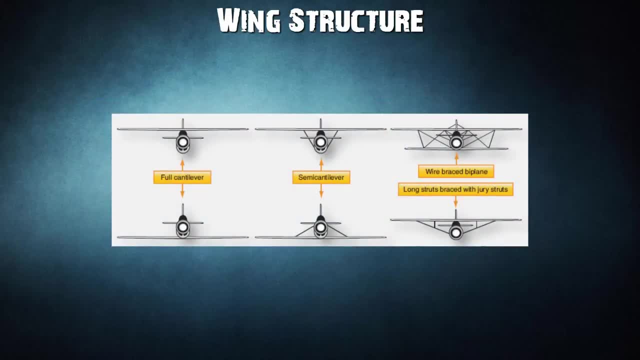 Other aircraft wings use external bracing struts or wires to assist in supporting the wing and carrying the aerodynamic and landing loads. wing support cables and struts are generally made from steel. many struts and their attach fittings have fairings to reduce, drag short nearly vertical supports, called jury struts. 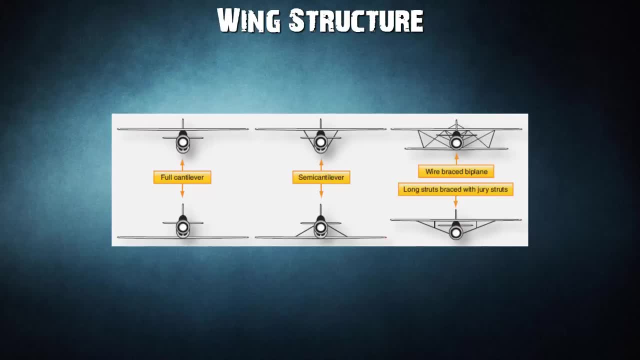 are found on struts that attach to the wings a great distance from the fuselage. this serves to subdue strut movement and oscillation caused by the air flowing around the strut in flight. the figure here shows samples of wings using external bracing, also known as semi Cantilever. 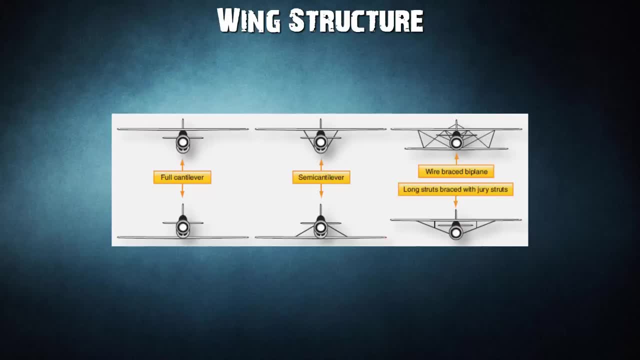 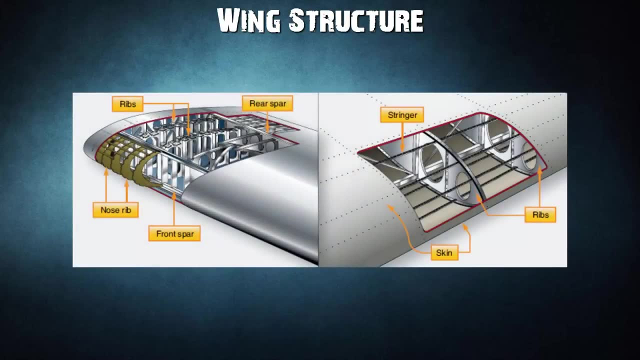 wings. Cantilever wings built with no external bracing are also shown. aluminum is the most common material from which to construct wings, but they can be wood covered with fabric. fabric and occasionally a magnesium alloy has been used. Moreover, modern aircraft are tending toward lighter and stronger materials throughout. 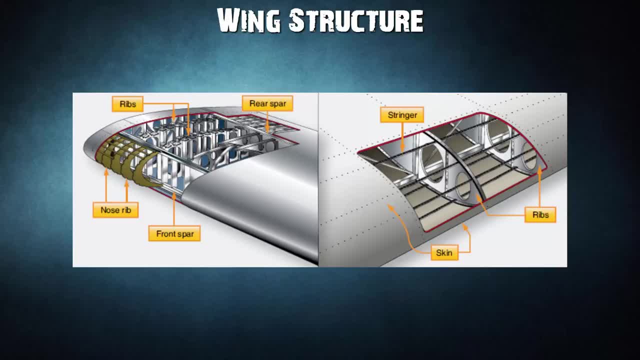 the airframe and in wing construction. Wings made entirely of carbon fiber or other composite materials exist, as well as wings made of a combination of materials for maximum strength to weight performance. The internal structures of most wings are made up of spars and stringers running spanwise. 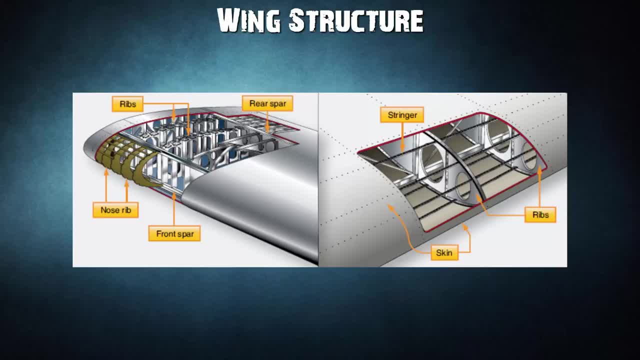 and ribs, and formers or bulkheads running cordwise leading edge to trailing edge. The spars are the principal structural members of a wing. They support all distributed loads as well as concentrated weights such as the fuselage, landing gear and engines. 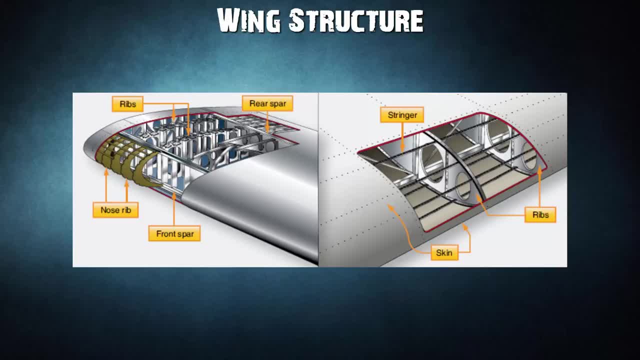 The skin, which is attached to the wing structure, carries part of the loads imposed during flight. It also transfers the stresses to the wing ribs. The ribs in turn transfer the loads to the wing spars. In general, wing construction is based on one of three fundamental designs. 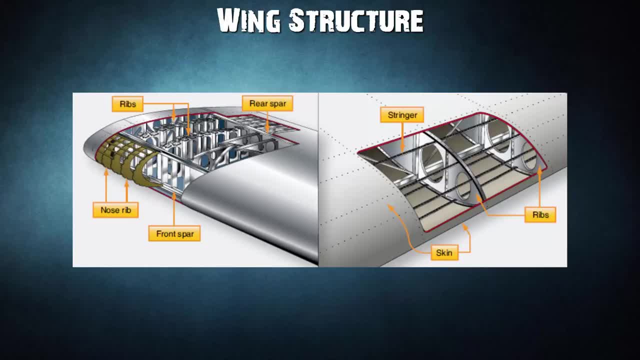 A, Mono spar B, Multi spar C Box beam. Modification of these basic designs may be adopted by various manufacturers. The mono spar wing incorporates only one main spanwise or longitudinal member in its construction. Ribs or bulkheads supply the necessary contour or shape to the airfoil. 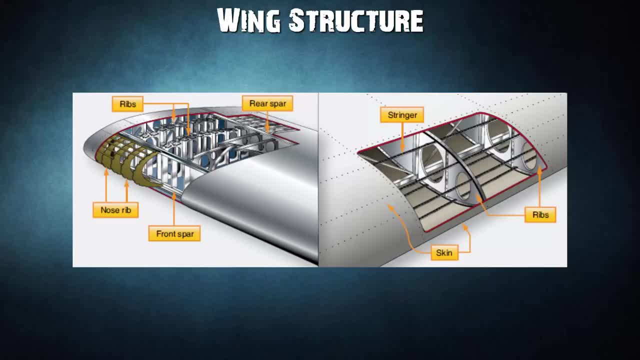 Although the strict mono spar wing is not common, the spars and stringers are often used in the construction of wings. This type of design, modified by the addition of false spars or light shear webs along the trailing edge for support of control surfaces, is sometimes used. 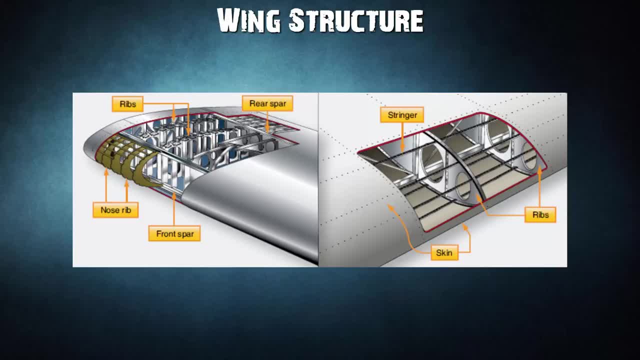 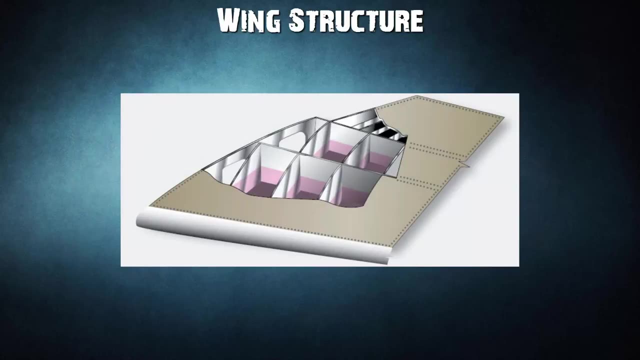 The multi spar wing incorporates more than one main longitudinal member in its construction. To give the wing contour, ribs or bulkheads are often included. The box beam type of wing construction uses two main longitudinal members with connecting bulkheads to furnish additional strength and to give contour to the wing. 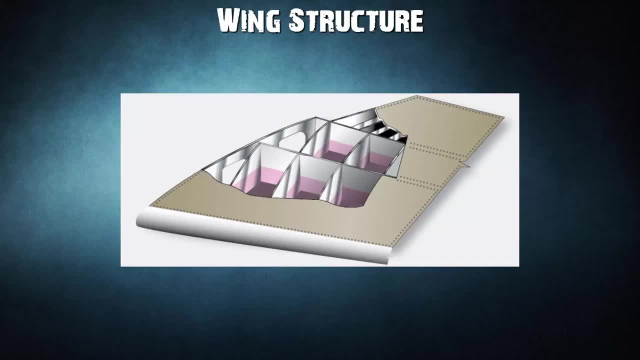 A corrugated sheet may be placed between the bulkheads and the smooth outer skin so that the wing can better carry tension and compression loads. In some cases, heavy longitudinal stiffeners are substituted for the corrugated sheets. The box beam type of wing construction uses two main longitudinal members with connecting bulkheads to furnish additional strength and to give contour to the wing. 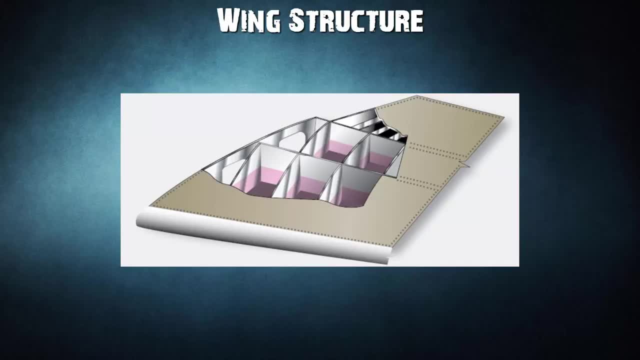 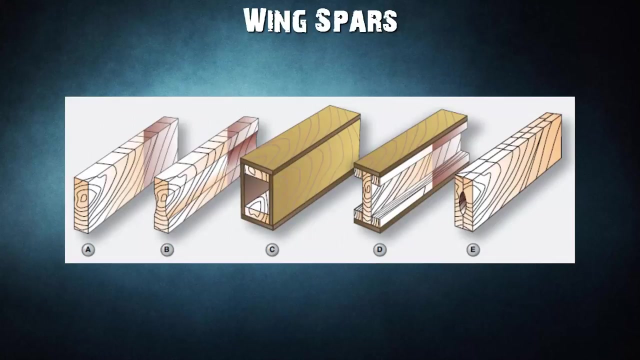 This combinedっ a combination of corrugated sheets on the upper surface of the wing and stiffeners on the lower surface is sometimes used. Air transport category aircraft often utilize box beam wing construction lease spars. Spars are the principal structural members of the wing. 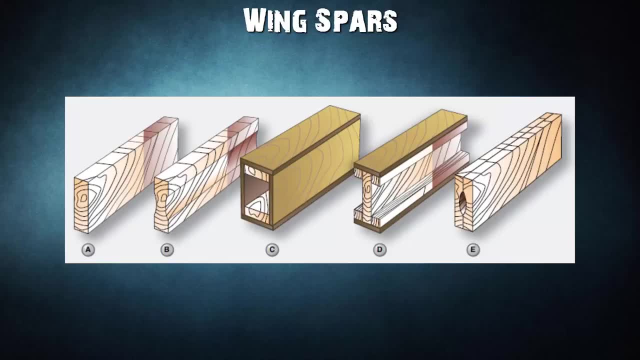 They correspond to the check the long airons of the fuselage. they run parallel to the lateral axis of the aircraft, from the fuselage toward the tip of the wing, and are usually attached to the fuselage by wing fittings, plane beams or a truss. spars may be made of metal, wood or composite materials, depending on the 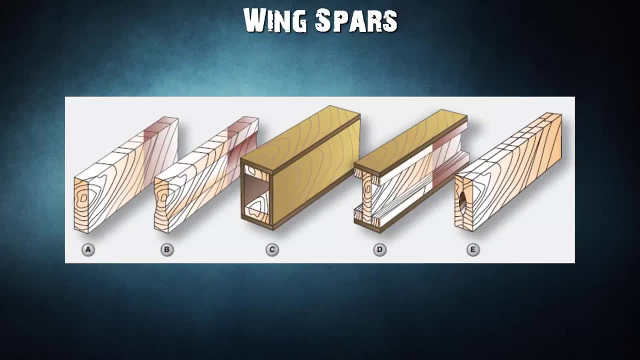 design criteria of a specific aircraft. wooden spars are usually made from spruce. they can be generally classified into four different types by their cross-sectional configuration, as shown here. they may be a solid be box shaped, see partly hollow, or D in the form of an I beam. 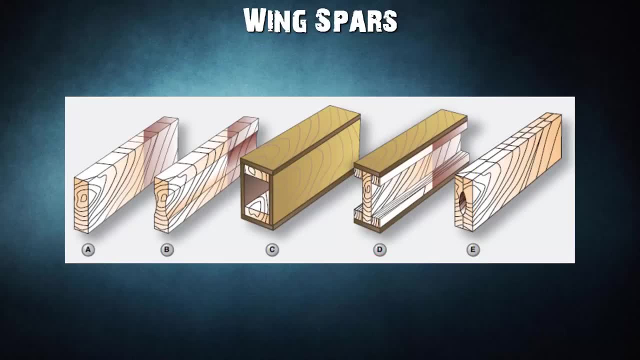 lamination of solid wood spars is often used to increase strength. laminated wood can also be found in box shaped spars. the e spar in the figure has had material removed to reduce weight but retains the strength of a rectangular spar. as can be seen, most wing spars are basically rectangular in shape, with the 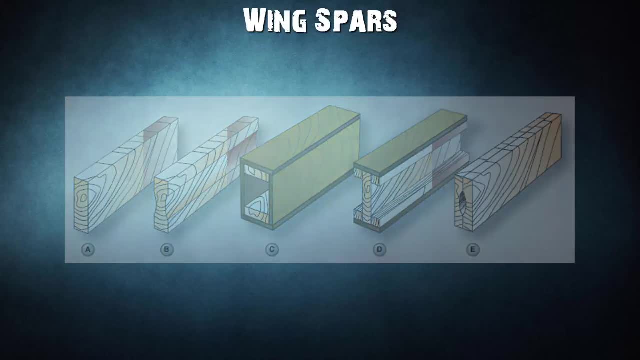 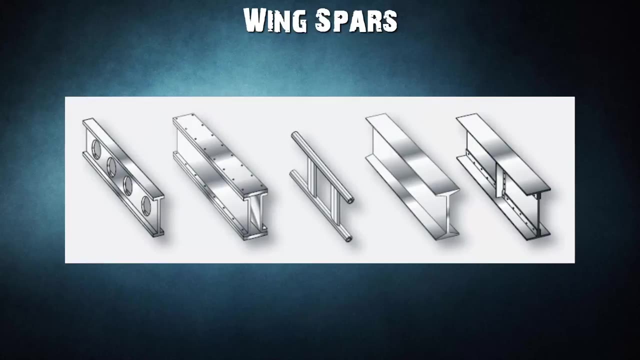 long dimension of the cross-section, oriented up and down in the wing. currently, most manufactured aircraft have wing spars made of solid extruded aluminum or aluminum extrusions riveted together to form the spar. the increased use of composites and the combining of materials should make airmen vigilant. 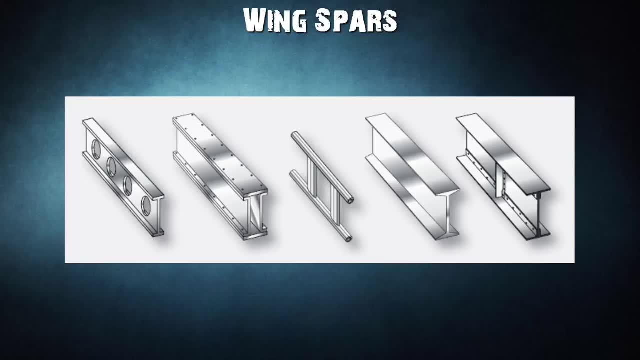 for wings spars made from a variety of materials. this figure shows examples of metal wing spar cross-sections. in an I beam spar, the top, you and bottom of the I beam are called the caps and the vertical section is called the web. the entire spark can be extruded from one piece of metal, but often it is. 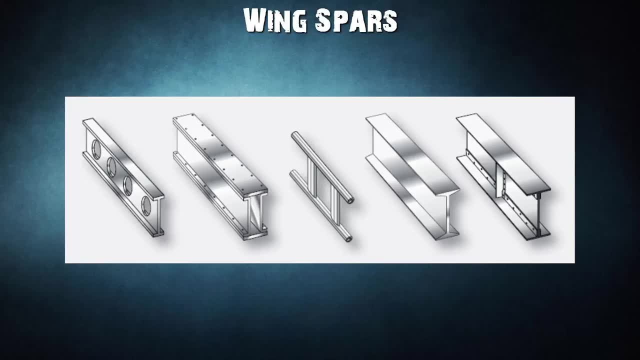 built up from multiple extrusions or formed angles. the web forms the principal depth portion of the spar, and the cap strips, extrusions, formed angles or milled sections are attached to it together. these members carry the loads caused by the wing spars as shown in the video. 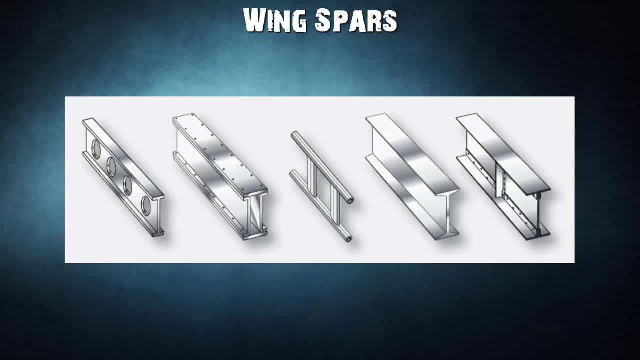 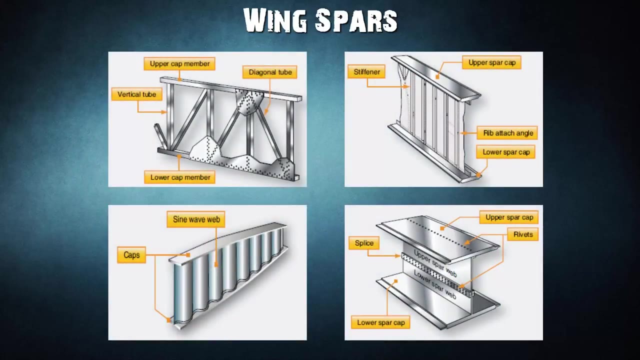 as shown in the video, by wing bending with the caps providing a foundation for attaching the skin. although the spar shapes are typical, actual wing spar configurations assume many forms. for example, the web of a spar may be a plate or a truss, as shown here. it could be built up from lightweight materials with vertical stiffeners. 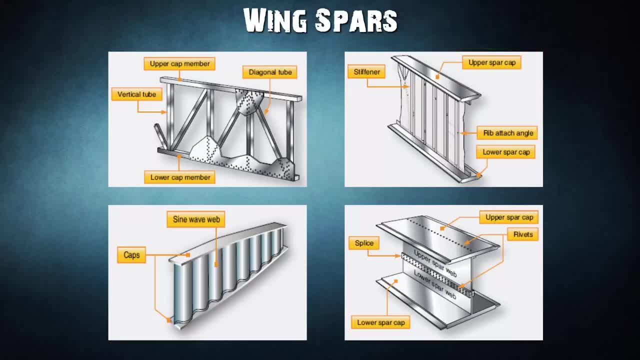 employed for strength, as shown here. as shown in the video, it could also have no stiffeners but might contain flanged holes for reducing weight but maintaining strength. some metal and composite wing spars retain the I beam concept but use a sine wave web. additionally, failsafe spar web design exists. failsafe means that should one. 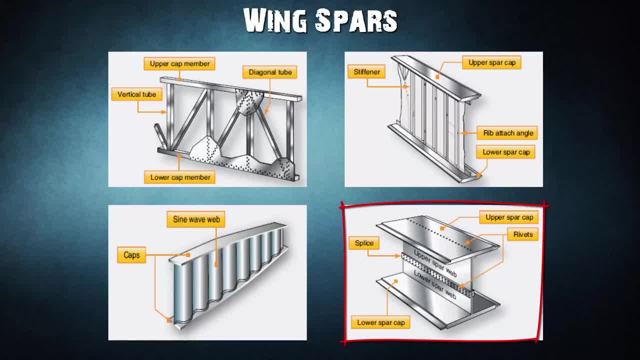 member of a complex structure fail, some other part of the structure assumes the load of the failed member and permits continued operation. a spar with failsafe construction is shown in this figure. this spars made in two sections. the top section consists of a cap riveted to the upper web plate. 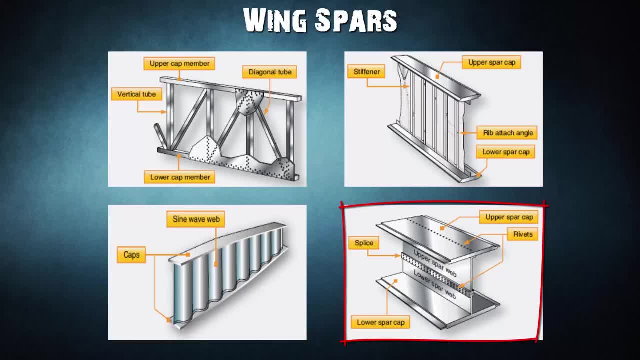 the lower section is a single extrusion consisting of the lower cap in web plate. these two sections are spliced to give her to form the first edge of the lower cap, we to form the spar. If either section of this type of spar breaks, the other section can. 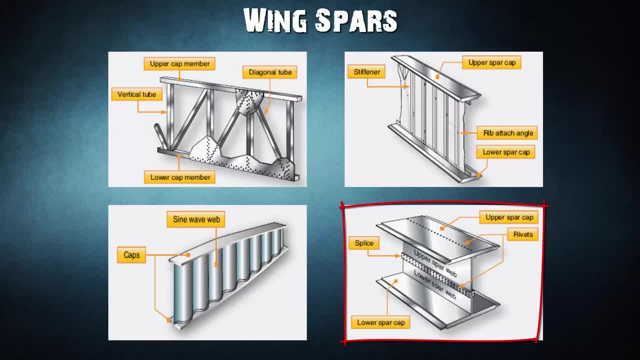 still carry the load. This is the fail-safe feature. As a rule, a wing has two spars. One spar is usually located near the front of the wing and the other about two-thirds of the distance toward the wing's trailing edge, Regardless, 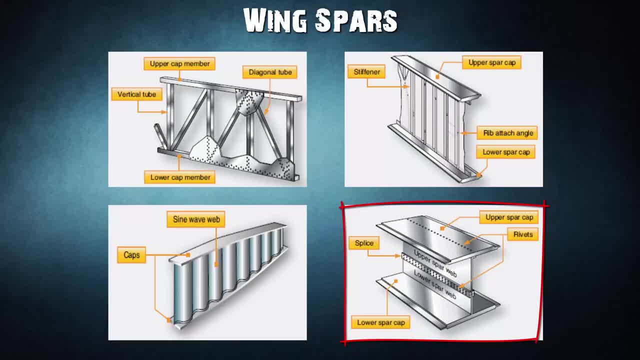 of the soft type, the spar is the most important part of the wing. When other structural members of the wing are placed under load, most of the resulting stress is passed on to the wing spar. False spars are commonly used in wing design. They are longitudinal members like spars, but 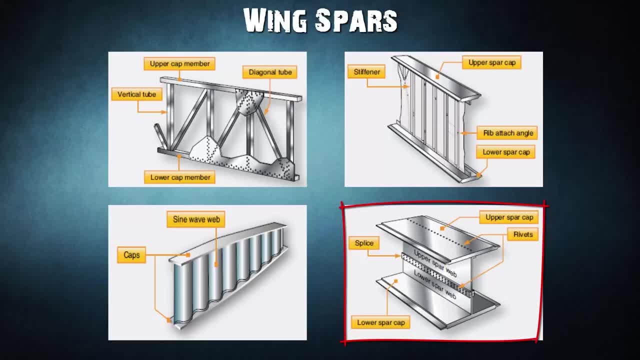 do not extend the entire spanwise length of the wing. Often they are used as hinge attach points. ibaWing comes in Mulloo wings in noise manuallycedes, stringed spars, リа Dong, monogluos and in astrowscarblurl similar to wontopinstrictions. 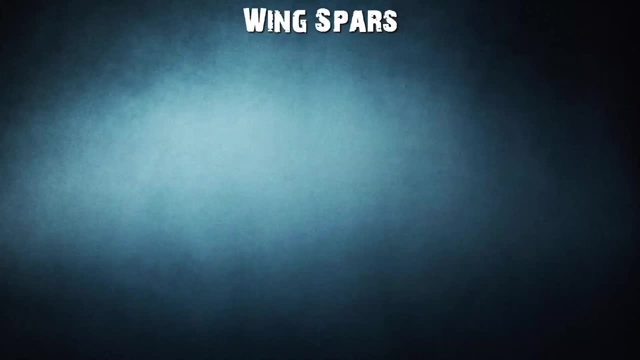 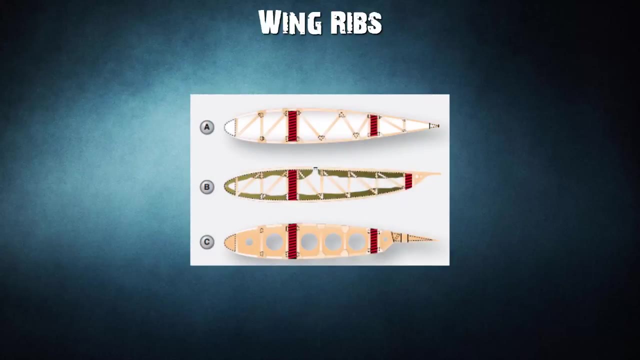 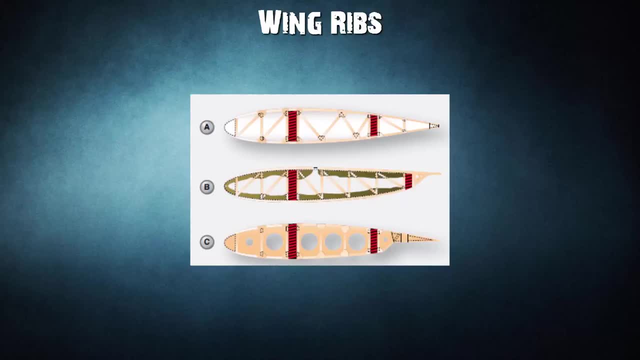 stringers to the spars. Similar ribs are also used in ailerons, elevators, rudders and stabilizers. Wing ribs are usually manufactured from either wood or metal. Aircraft with wood wing spars may have wood or metal ribs, while most aircraft with metal spars. 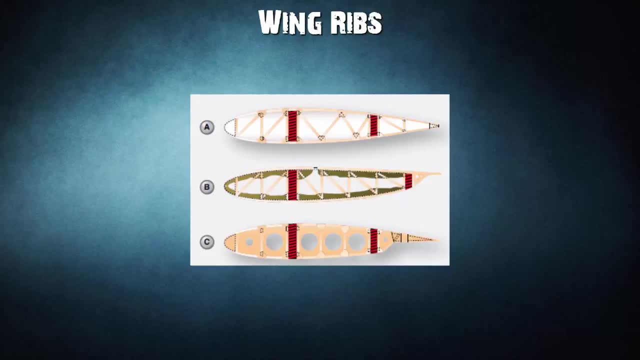 have metal ribs. Wood ribs are usually manufactured from spruce. The three most common types of wooden ribs are the plywood web, the lightened plywood web and the truss types. Of these three, the truss type is the most efficient because it is strong and lightweight, but it is also the most complex. 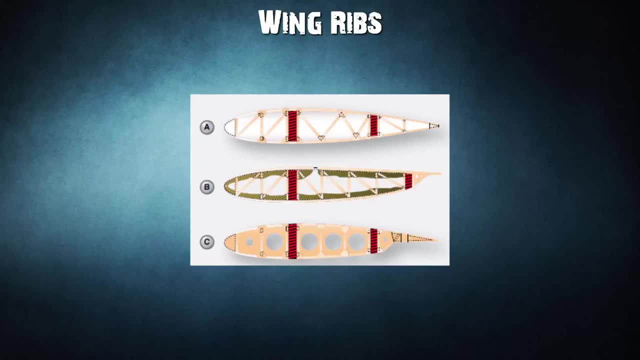 to construct. This figure is the most. The figure shows wood truss web ribs and a lightened plywood web rib. Wood ribs have a rib cap or cap strip fastened around the entire perimeter of the rib. It is usually made of the same material as the rib itself. 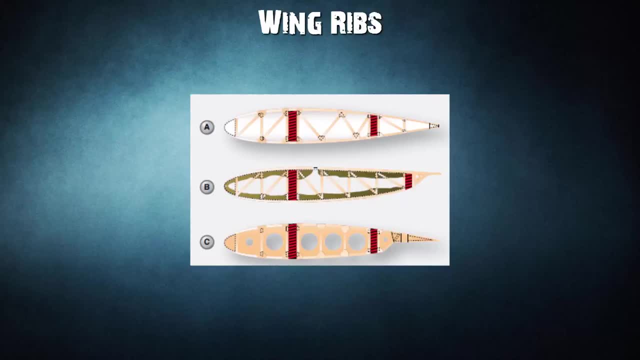 The rib cap stiffens and strengthens the rib and provides an attaching surface for the wing covering. In figure A, the cross section of a wing rib with a truss type web is illustrated. The dark rectangular sections are the front and rear wing spars. 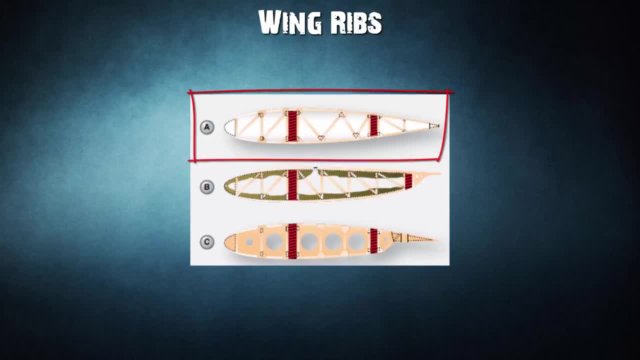 Note that to reinforce the truss gussets are used. In figure B a truss web rib is shown with a continuous gusset. It provides greater support throughout the entire rib with very little additional weight. A continuous gusset stiffens. 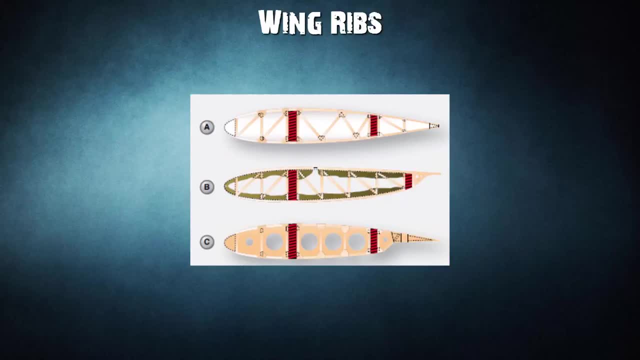 the cap strip in the plane of the rib. This helps to prevent buckling and helps to obtain better rib slash skin joints where nail gluing is used. Such a rib can resist the driving force of nails better than the other types. Note that continuous gussets are also more easily handled than the many small separate. 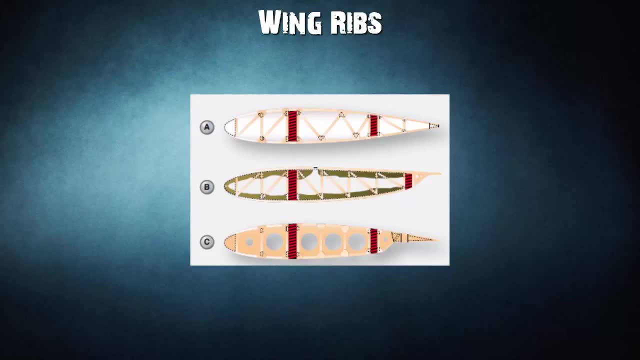 gussets otherwise required. Figure C shows a rib with a lightened plywood web. It also contains gussets to support the web-slash-cap-strip interface. The cap strip is usually laminated to the web, especially at the leading edge. 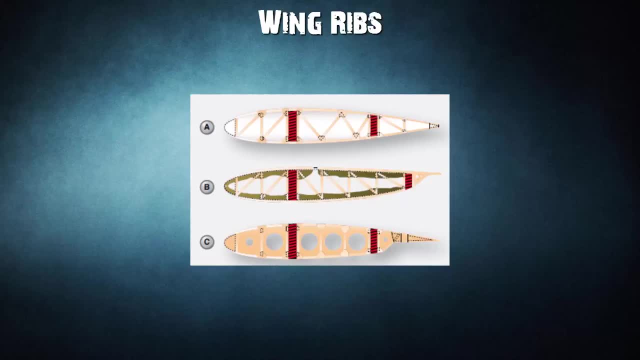 A wing rib may also be referred to as a plain rib or a main rib. Wing ribs with specialized locations or functions are given names that reflect their uniqueness. For example, ribs that are located entirely forward of the front spar, that are used to shape and strengthen the wing leading edge, are called nose ribs or false ribs. 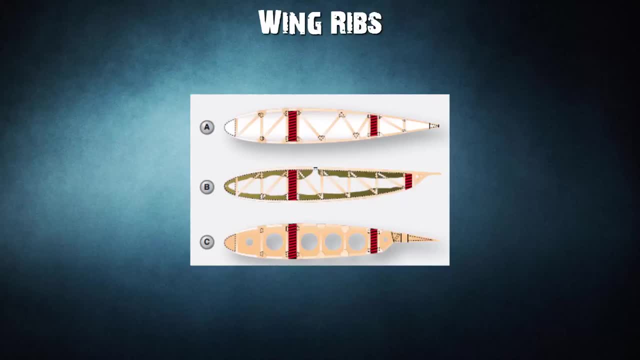 False ribs are ribs that do not span the entire wing cord, which is the distance from the leading edge to the trailing edge of the wing Wing. butt ribs may be found at the inboard edge of the wing, where the wing attaches to the fuselage. 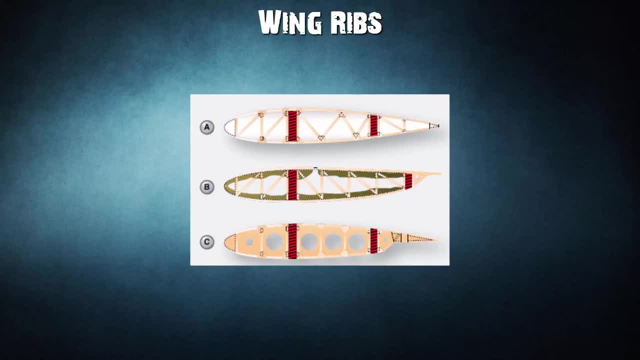 Depending on the wing's shape. the wing may be shaped as a wing rib. Depending on its location and method of attachment, a butt rib may also be called a bulkhead rib or a compression rib if it is designed to receive compression loads that tend to force the wing spars together. 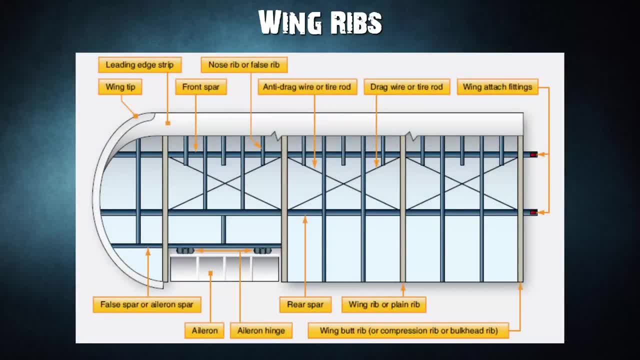 Since the ribs are laterally weak, they are strengthened in some wings by tapes that are woven above and below rib sections to prevent sidewise bending of the ribs. Drag and anti-drag wires may also be found in a wing. In this figure they are shown criss-crossed between the spars to form a truss to resist forces acting on the wing in the direction of the wing cord. 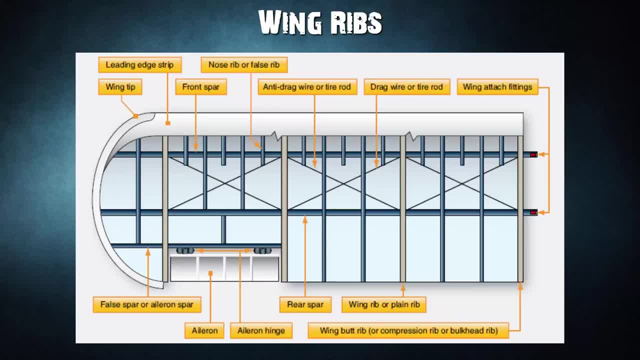 These tension wires are also referred to as tie rods. The wire designed to resist the backward forces is called a drag wire. The anti-drag wire resists the forward forces in the cord direction. Figure also illustrates the structural difference. The These provide a strong and secure method for attaching the wing to the fuselage. 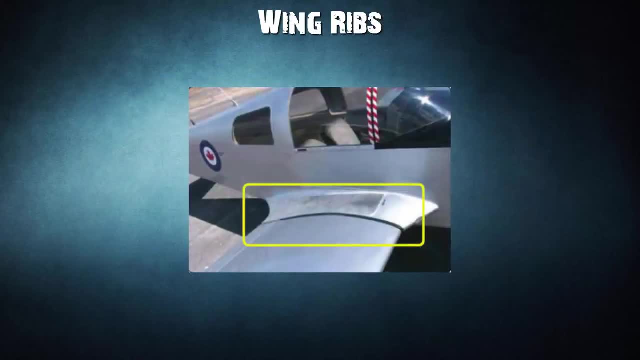 The interface between the wing and fuselage is often covered with a fairing to achieve smooth airflow. in this area, The fairings, as shown in this figure, are used to attach the wing to the fuselage. The wing tip, as shown in this figure, can be removed for access to the wing attach fittings. 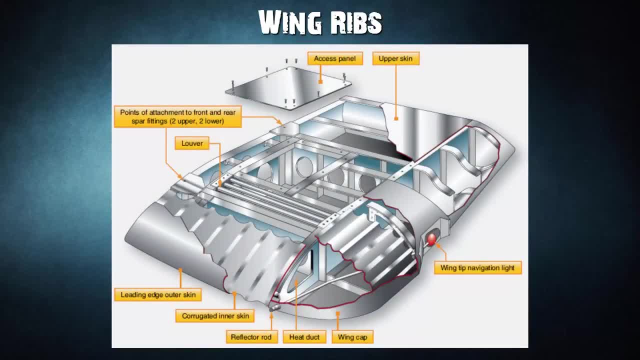 The wing tip is often a removable unit bolted to the outboard end of the wing panel. One reason for this is the vulnerability of the wing tips to damage, especially during ground handling and taxiing. Here is a removable wing tip for a large aircraft wing. 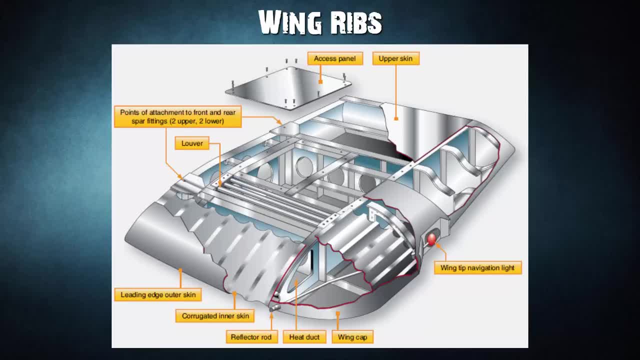 others are different. the wingtip assembly is a voluminum alloy construction. the wingtip cap is secured to the tip with countersunk screws and is secured to the inter spar structure at four points with quarter of inch diameter bolts to prevent ice from forming on the leading edge. 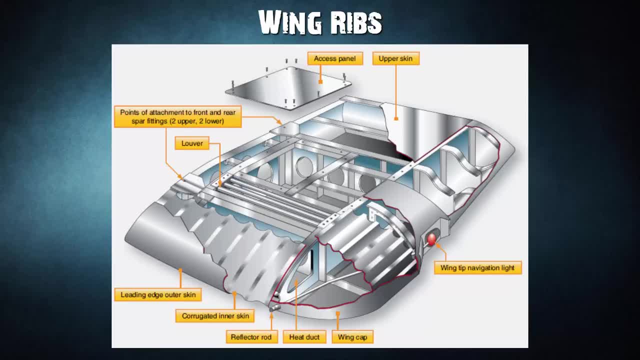 of the wings of large aircraft. hot air from an engine is often channeled through the leading edge from wing route to wingtip. a louver on the top surface of the wingtip allows this warm air to be exhausted. overboard. wing position lights are located at the center of the tip and are 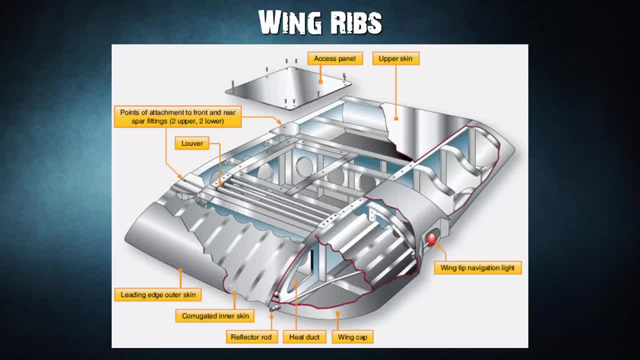 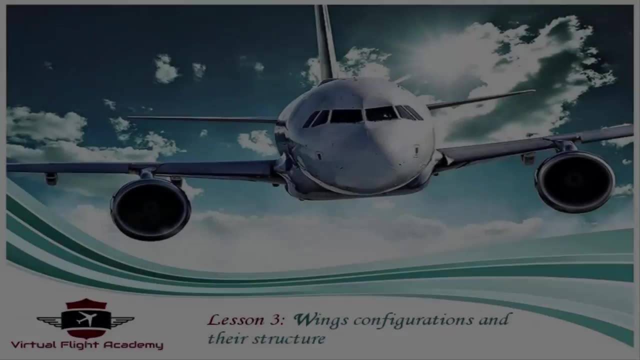 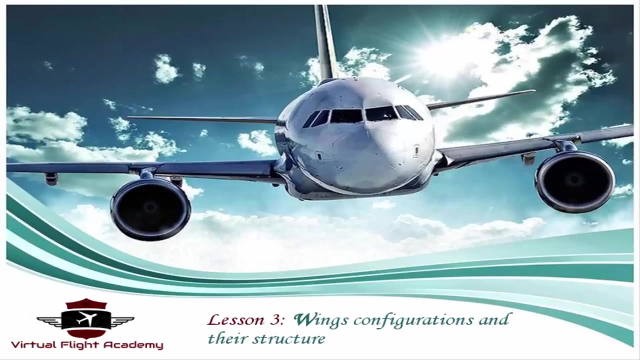 not directly visible from the cockpit as an indication that the wingtip light is operating. some wingtips are equipped with a lucite rod to transmit the light to the leading edge. this is the end of part 1 in lesson 3. if you learned something, please click the. 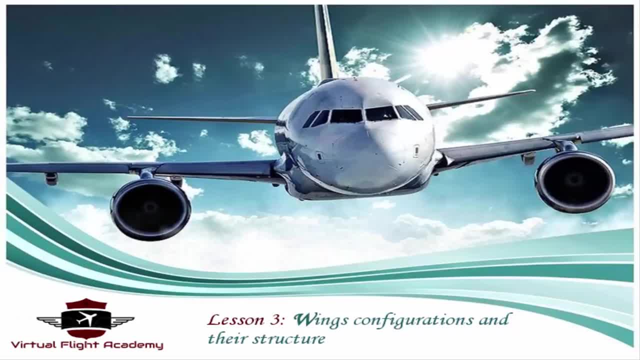 like button and subscribe to our channel and stay tuned for part 2.